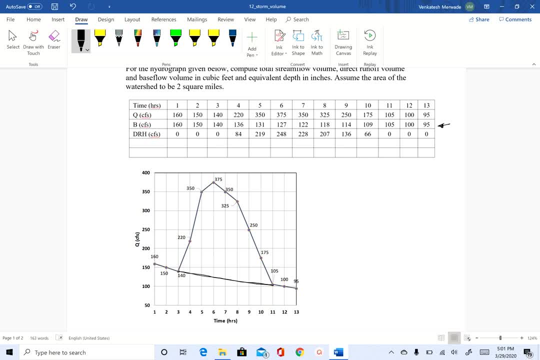 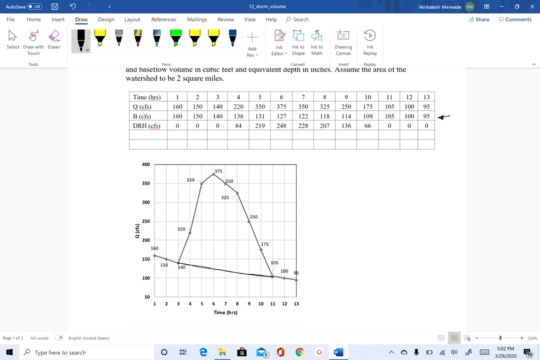 Now don't use the values that I have given you here for assignment 11, because I did round up some of these numbers, So let's see how we can get the total volume. So this is simple geometry and math, and you have done this in one of your homework problems, but I still wanted to make this video so you can come back to this whenever we are going to calculate the stream flow volume- and we will be doing this for quite a few times- when we are going to look at the unit hydrographs. 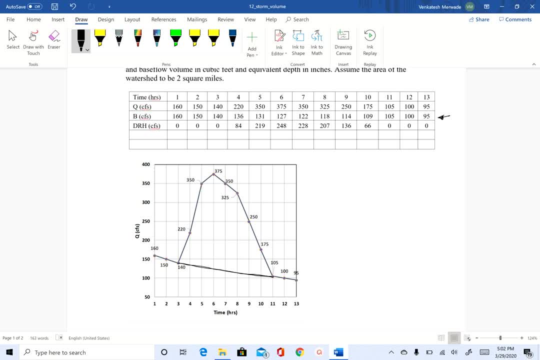 So to get the total volume, we need to calculate the stream flow volume. So to get the total volume, what we need is the area under this curve. So one way to do that is to divide this curve into these trapezoids. I'll just use a different color here. 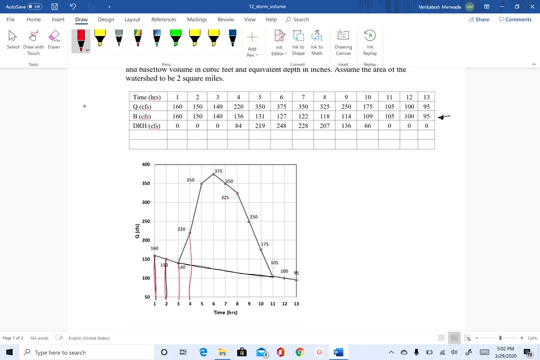 So all I'm doing here is dividing the stream flow hydrograph into these trapezoids, and then I will just calculate the area for each trapezoid. So what we need is the area under this curve. So what we need is the area under this curve. 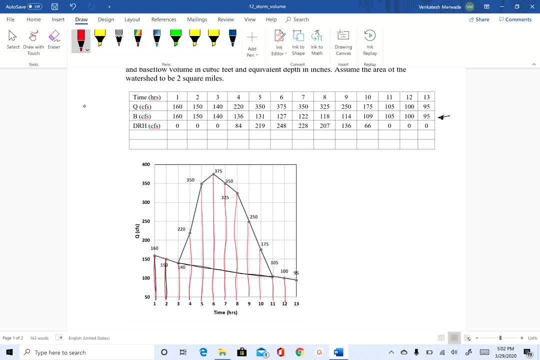 So what I will do is I will just do this for the first two trapezoids and then you can do the rest. So let me start with the first one. So for this, the area is going to be 160 plus 150 divided by 2 times the height, or in this case it will be delta t, which is one hour. 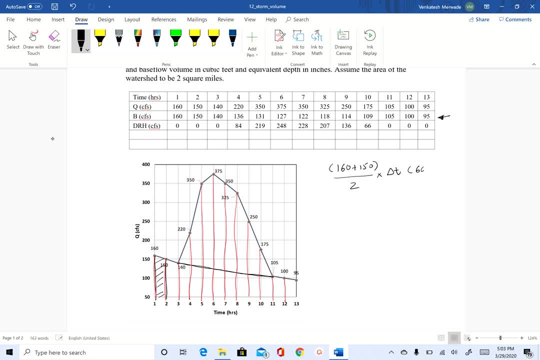 So instead of delta t, it will be 1 hour. So, instead of delta t, it will be 1 hour. So instead of delta t, it will be 1 hour. So instead of delta t, you need 60 times 60, which is 60 seconds in 60 minutes. 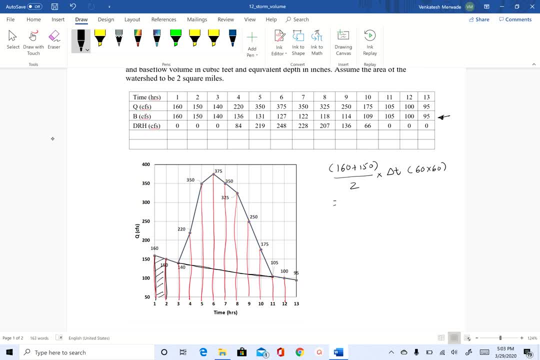 So if you do that, what you get is 558, 10 to the power of 3 cubic feet. So I can now write base flow volume or no. that's the total volume. So total volume in 10.. So total volume in 10 to the power of 3.. 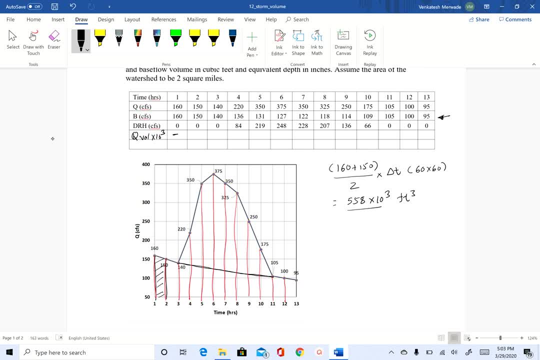 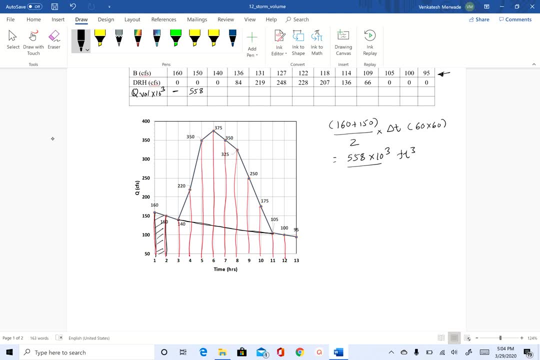 So I will keep this blank. So this will be 558.. Similarly, let's do one more for this video and then you can do the rest. So for this trapezoid, this is going to be 150 plus 140, divided by 2 times 3600.. 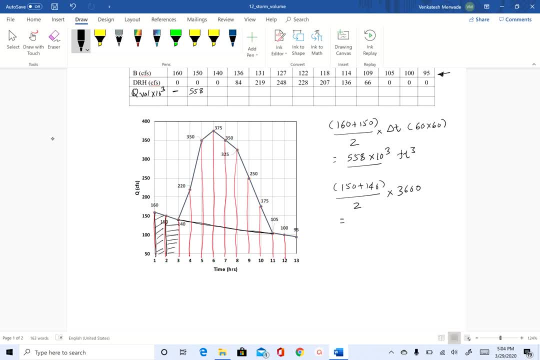 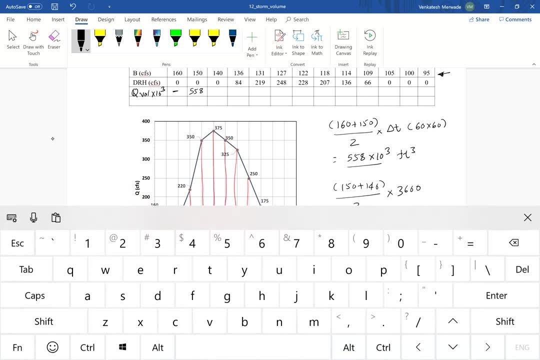 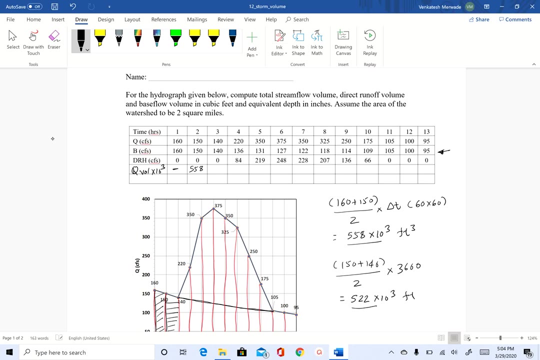 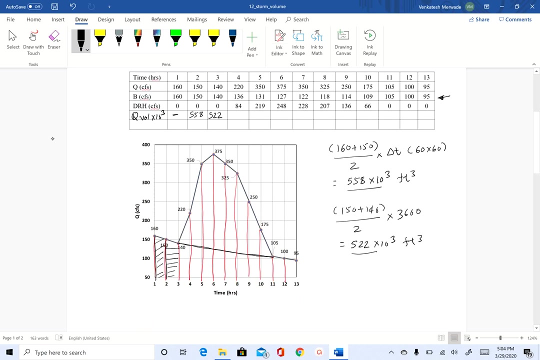 And if you do that, what you get? So let me write that again. So the total volume that I get in three years what I get is 522, 10 to the power of three cubic feet. So I'll write that down here: 522, and you can do the rest okay. 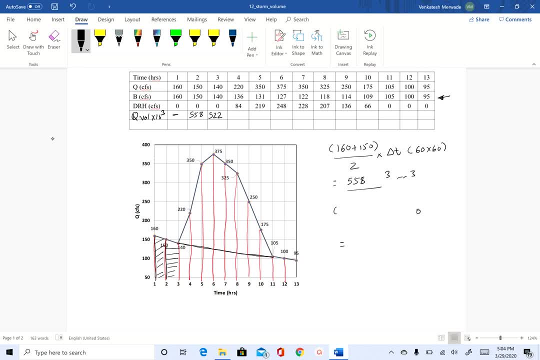 So I have done all this. Okay, So I have done all this And the total: Okay, So I have done all this and the total, So I have done all this and the total volume that I get for the streamflowámof20m. 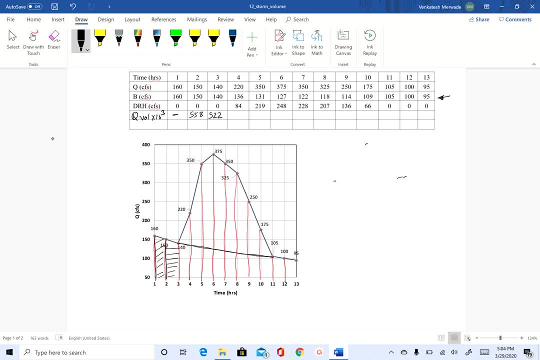 is so Q total that I get is nine point six ten to the power of six cubic feet. okay, so this is how we got the, the volume for the total stream flow, which was to divide the entire hydrograph into these trapezoids. now to get the base. 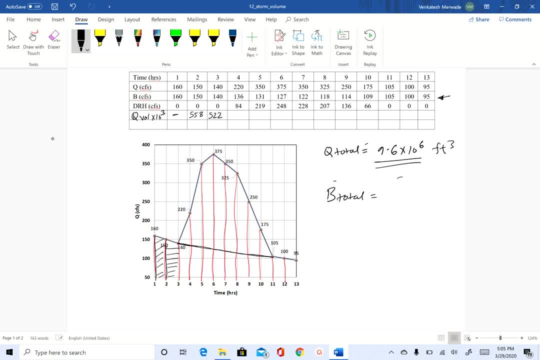 flow. all you have to do is you have to remain under this line. so what I can do is I can remove all these other lines and maybe use a different color. so here we are going to get the area for these smaller trapezoids okay. so you can. 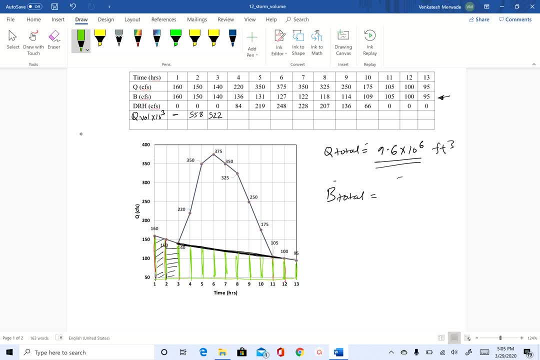 either do the this for each individual trapezoid or, if you think about it, there are only three trapezoids here, so, if you want, you can do this for each individual, or you can just do this for these three different colors that I'm showing here. I have 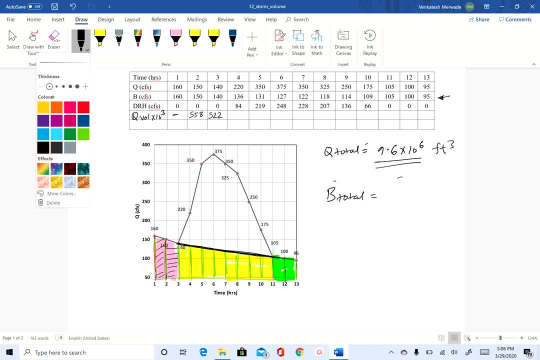 already done that for you. so if you do this correctly, the total volume that you should get is ten to this, five point three, three, ten to the power. oh, this should be five point three, three, ten to the power of six, and then to get the direct run of volume. 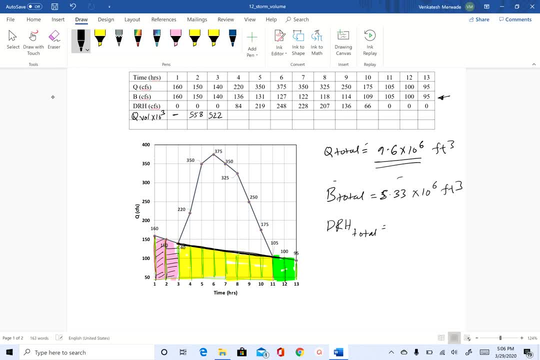 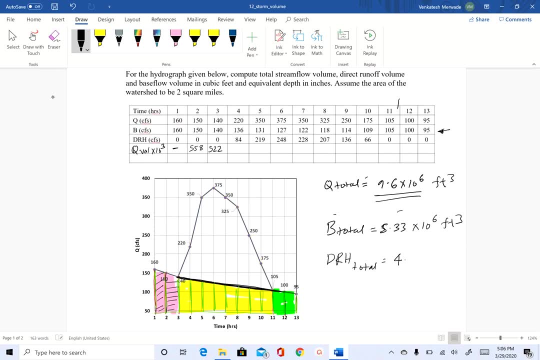 you subtract base flow from the total amount of volume in T 0 to get the base flow away from the total column of volume, and then you subtract back this flow and that gives you 4, 4.27, 10 to the power of 6 cubic feet. okay, so this is. 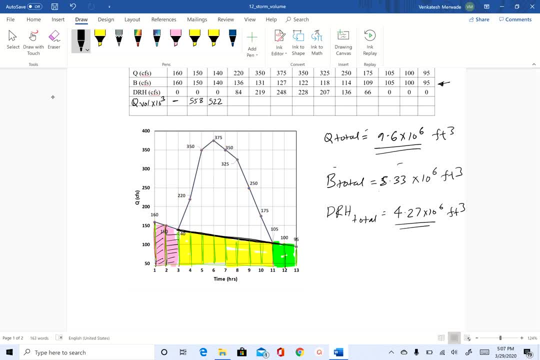 how you will get the the volume for the total stream flow, base flow and direct runoff. now, just by looking at this figure, you may wonder why. why we are getting higher volume for a base flow even though the area is small. remember we started at 50 here, not zero. so if I had plotted this from zero- the base flow- 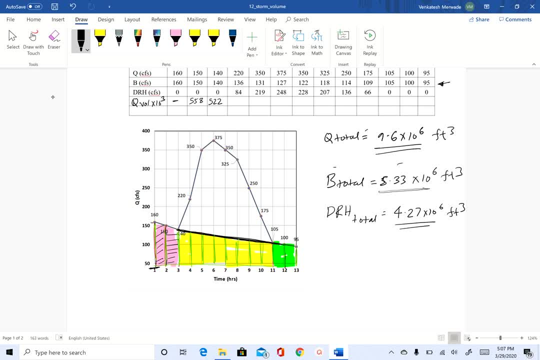 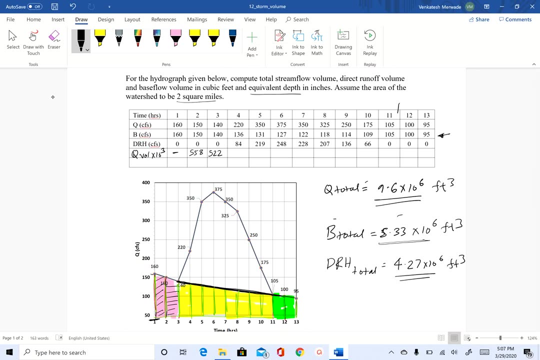 area is actually bigger than the direct runoff volume area. okay, so that's why our base flow number is higher than the direct runoff volume. so this is the volume in cubic feet. I have also asked you to get the equivalent depth if the watershed area is 2 square miles. 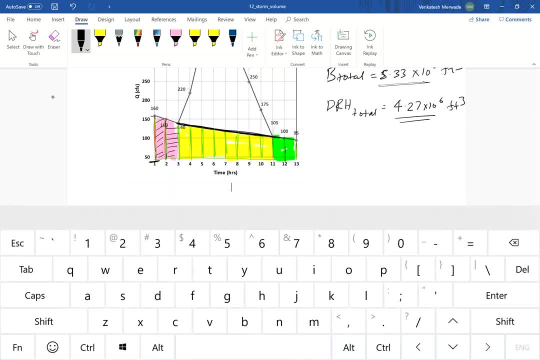 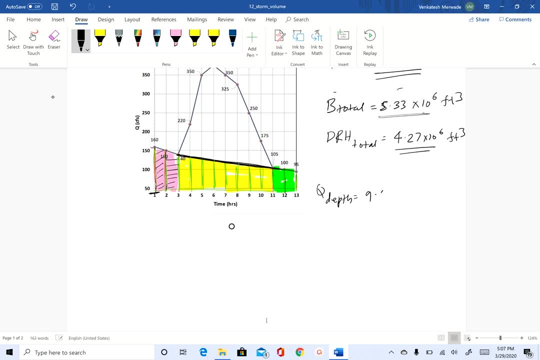 so this is the volume in cubic feet. I have also asked you to get the equivalent depth if the watershed area is 2 square miles. so so to do that, all you have to do is so let me just do this for Q depth. so we had nine point six, ten to the power of six. so that's the volume you divided by 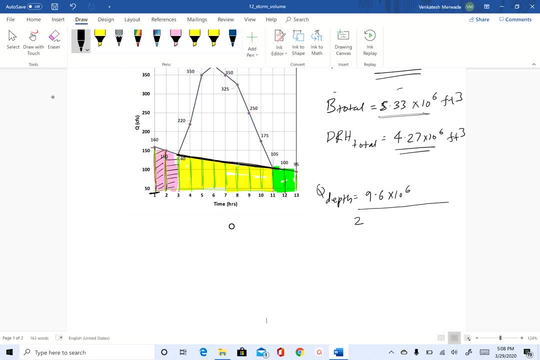 area. our area is two square miles and each mile is five to eight zero feet. so because we have square miles, I'll do this two times: five to eight zero, and if you do that, the number that you will get is zero point one, seven, two feet, okay. 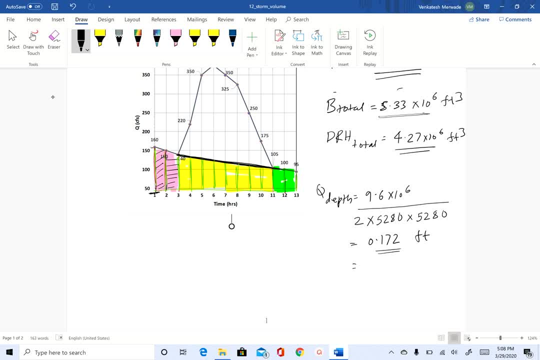 so we are talking about water depth here, so we usually do that in inch or centimeter. so I'm going to convert this feet into inches by multiplying it by 12, and if you do that, we end up with approximately two inch of water, or in this case, total stream flow depth, and if you do the same, you will get base flow. 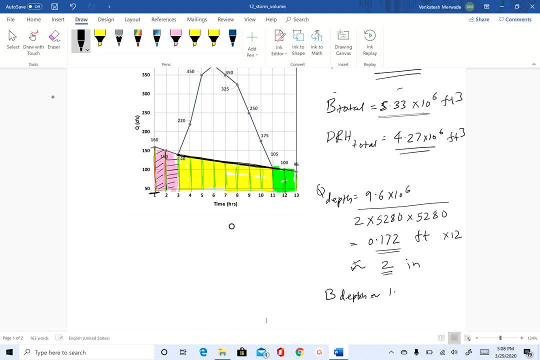 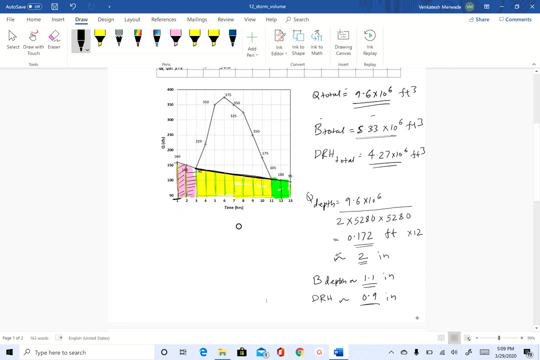 depth of approximately 1.1 inch and then the direct runoff depth of approximately 0.9 inch. okay, so this is how you can calculate the volume under this hydrograph, both in terms of cubic feet or meter cube, if the unit was in meter cube per second, and also you can get the equivalent depth, if you know. 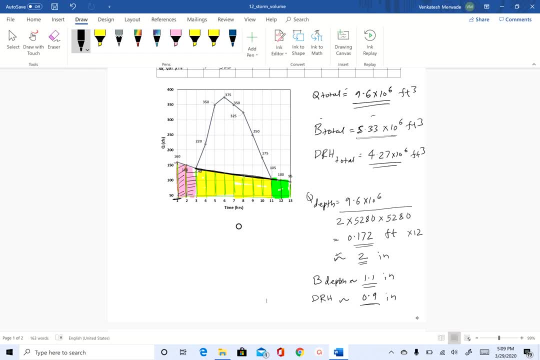 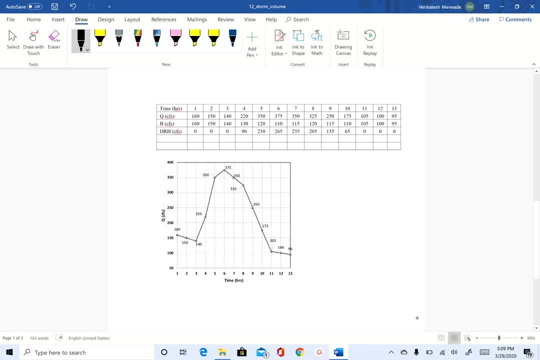 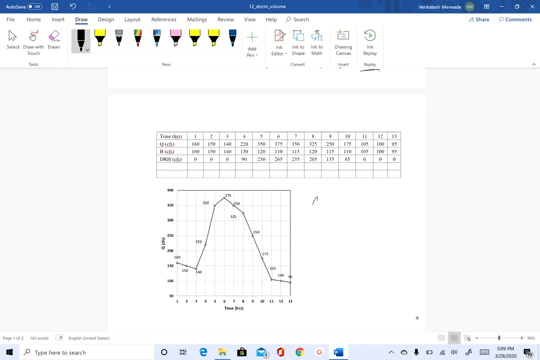 the area. okay, so remember this method. there is another page here in your assignment 12. so in this case I have given you base flow values by using the, the variable slope method. so go ahead and do the same calculations or similar calculation and get. So, in this case, Q total is not going to change, which is nine point six ten to the power of six cubic feet. 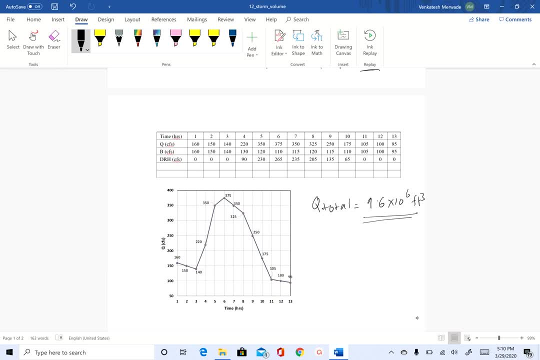 Your base flow value will change, so base flow total Will change. so that's something that you have to calculate, and direct runoff total Will also change, which is something that you will calculate. The reason I wanted to give this additional problem to you was to see the change in base flow. 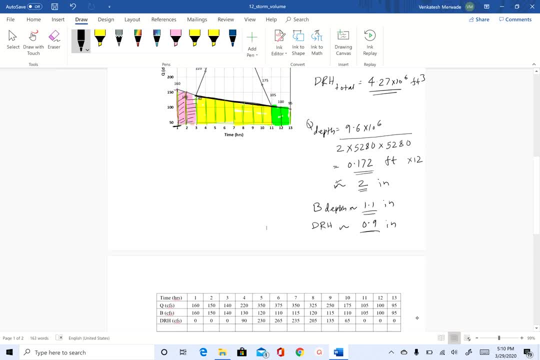 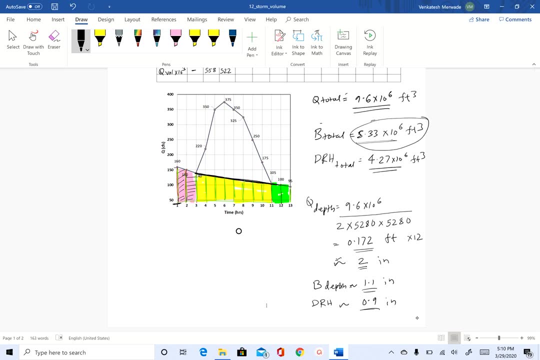 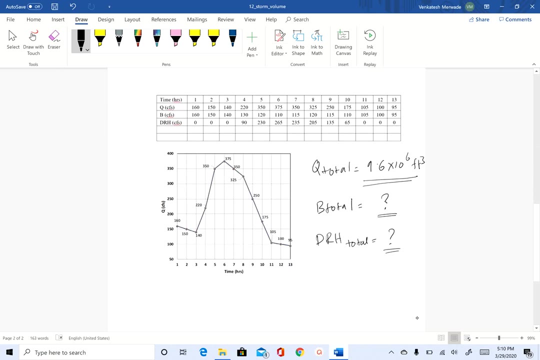 Volume when you use a different technique. So what you have done here in problem number one is to use the straight line method, and this is the volume you got, This is the depth you got. now do the same for this numbers, which was, Which were calculated using the variable slope method, and so 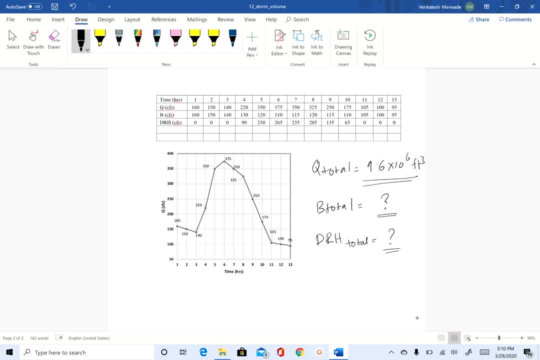 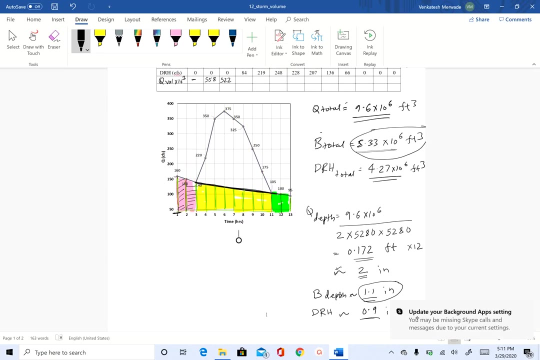 What values you get for the volume, for both base flow and direct runoff, both in terms of cubic feet and also in inch, and You can do these calculations on your own by using What we did for this problem. So I hope you were able to follow all my calculations and if you have any questions, 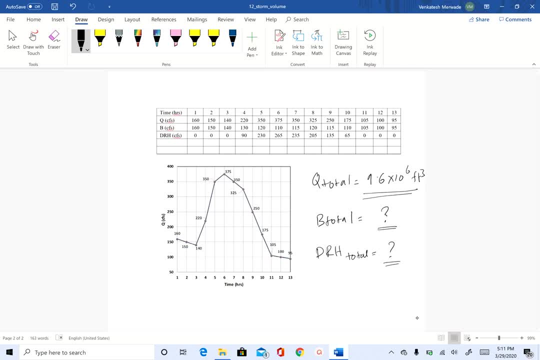 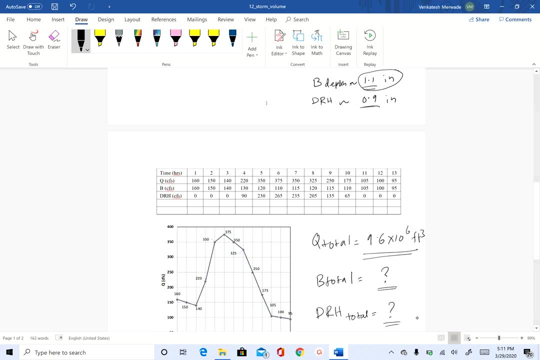 Feel free to email me, and this is it for assignment 12. so all the best and I'll see you in the next video. Thank you and bye. 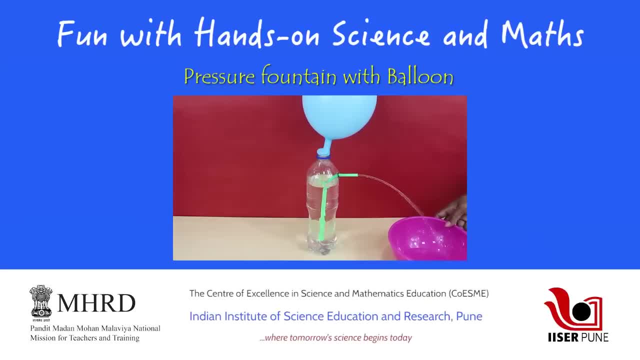 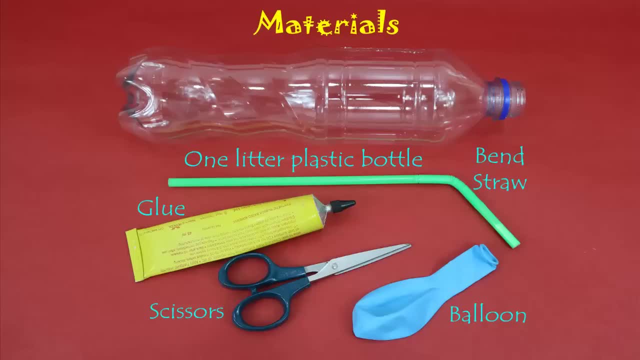 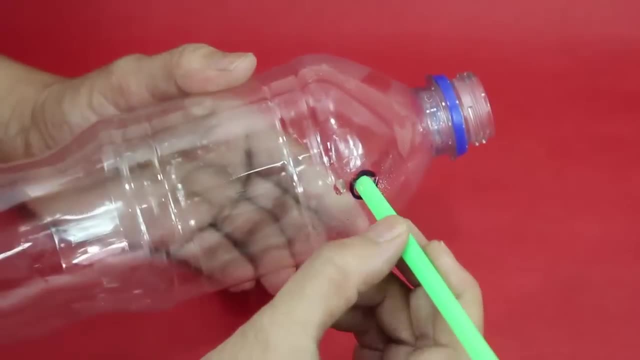 In this video you will learn to make a wonderful water fountain with very simple materials. For this you will need a balloon, a plastic bottle, a bendable straw glue and a pair of scissors. Make a hole near the mouth of the plastic bottle with scissors. 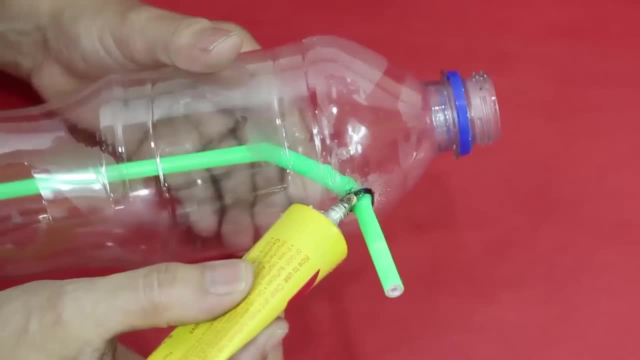 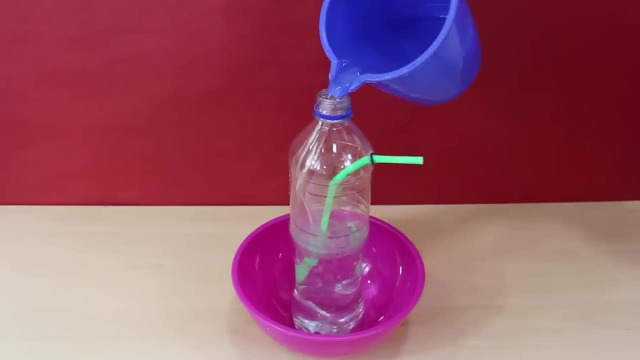 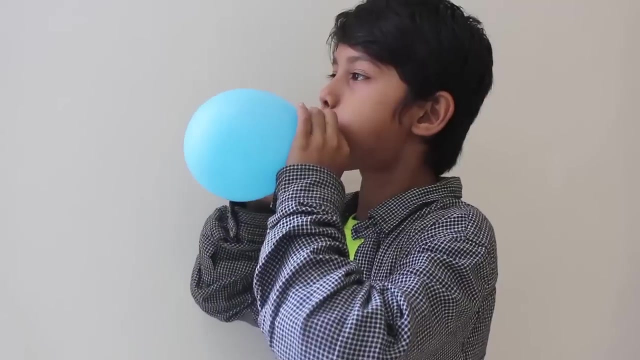 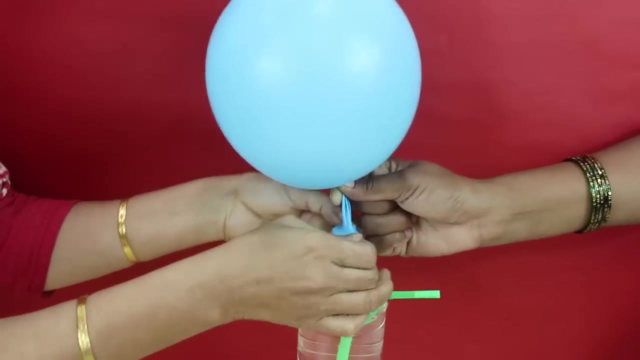 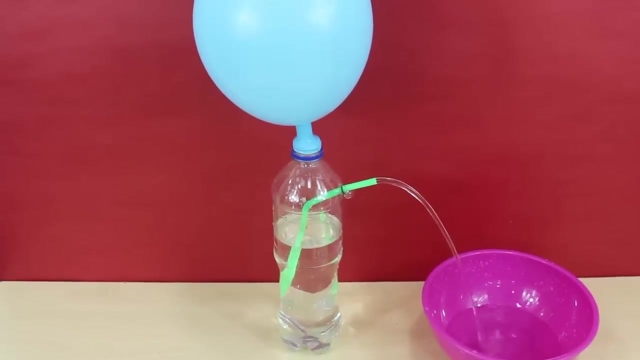 Insert a straw in the bottle and secure the hole with help of glue. Fill the bottle with water, Close it. Now blow a balloon and hold the neck Carefully. fix the balloon on the mouth of the bottle. When you release air from the ballon, it creates pressure in the bottle. 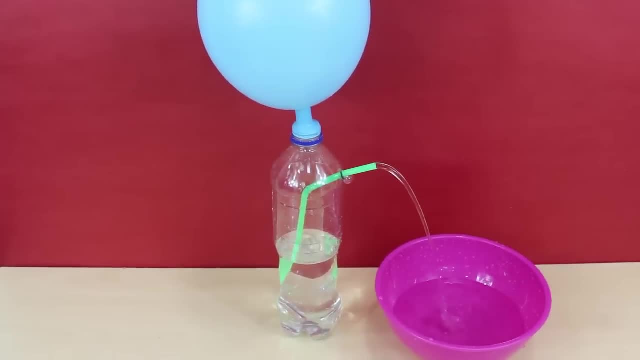 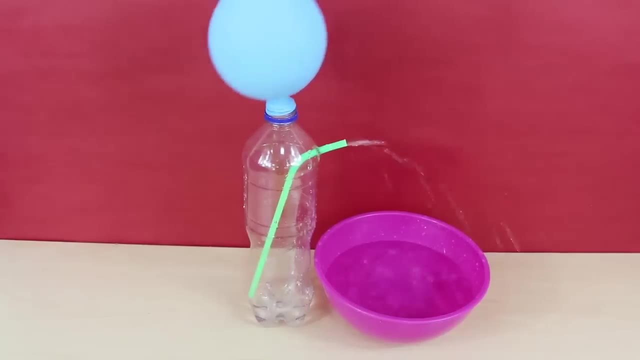 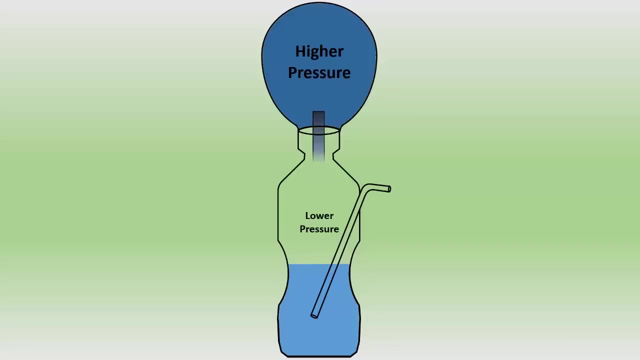 It also may push the water out, creating a water fountain. So lets look at what actually happens in this experiment. The air inside the balloon is under higher pressure. When you place the inflated balloon on the mouth of the bottle, the air pressure on the 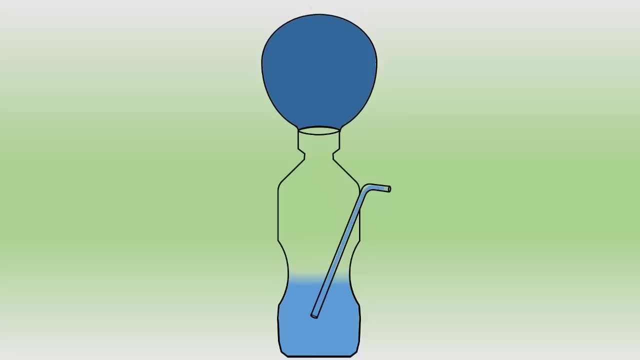 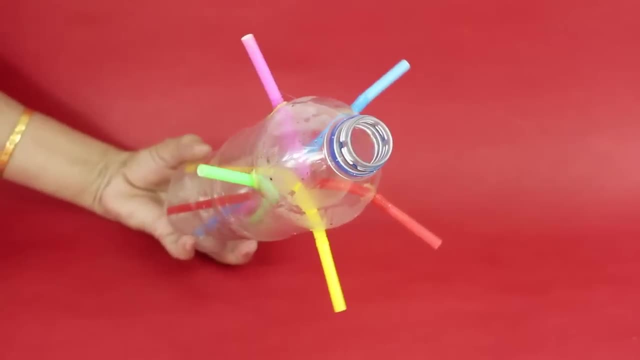 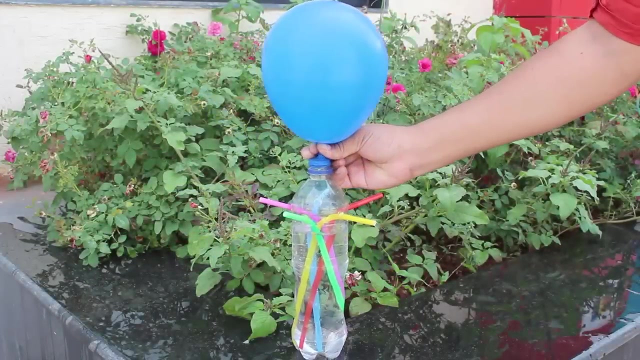 top of the bottle increases, This pushes down on the water in the bottle, which rises through the straw and comes out making a little fountain. Instead of a single straw, you can also fix 5 straws in the bottle. You can fill the water in the bottle and fix an inflated balloon. 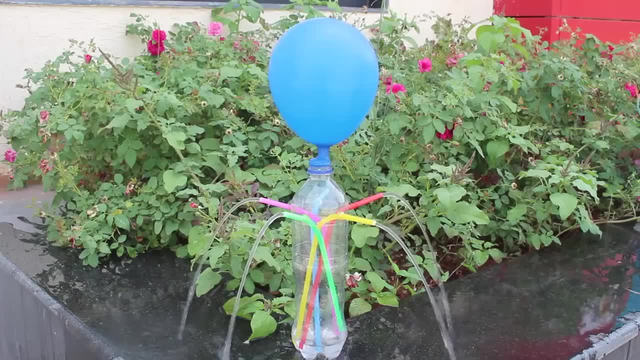 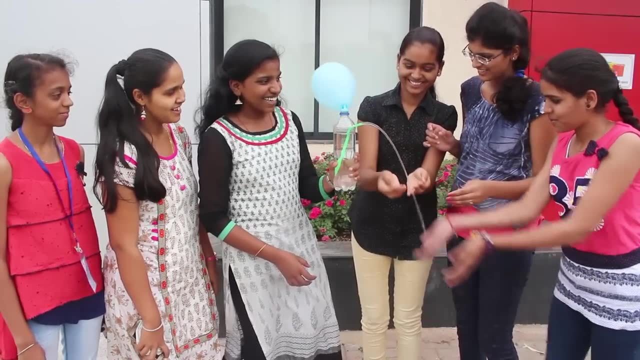 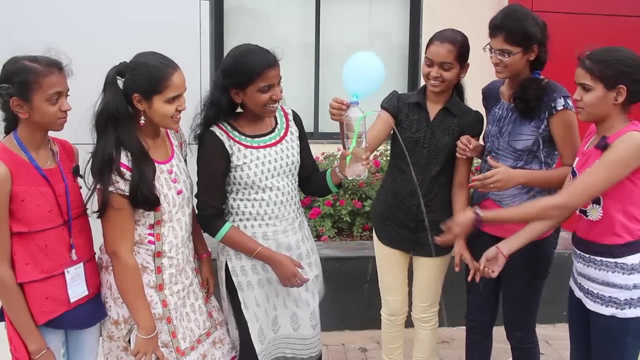 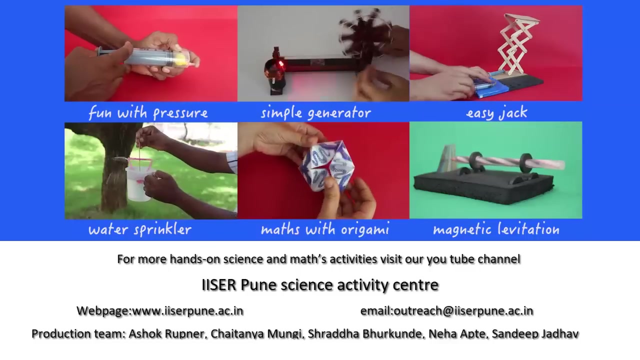 You will see an elegant fountain with 5 streams. Make your own pressure fountain and have fun. We hope you enjoyed this experiment and learnt something new today. For more such hands on science and mathematics activities, visit our YouTube channel: Iser Pune Science Activity Center.